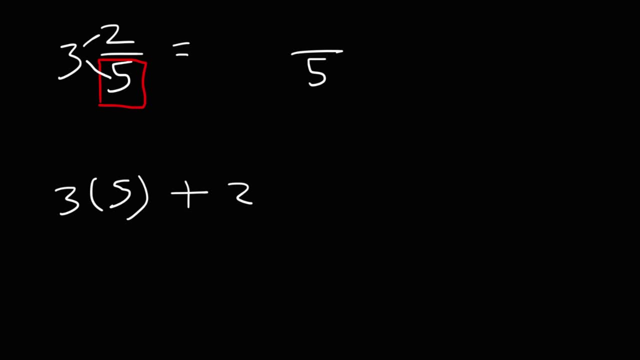 So I'm going to write that out: 3 times 5.. 3 times 5 plus 2.. 3 times 5 is 15.. 15 plus 2 is 17.. So that's how you can convert a mixed number into an improper fraction. 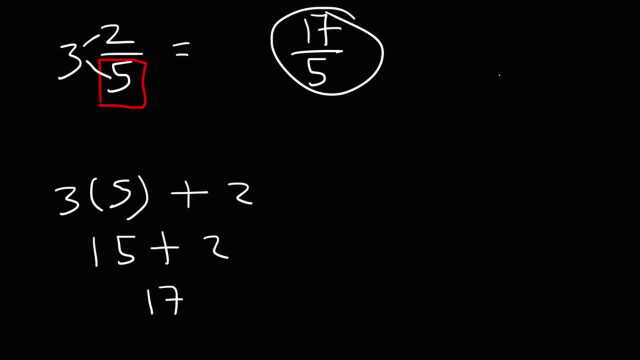 Now, once you have the improper fraction, you can flip it in order to get the reciprocal. So the reciprocal is going to be 5 over 17. And this is the answer. So that's how you can find a reciprocal of a mixed number. 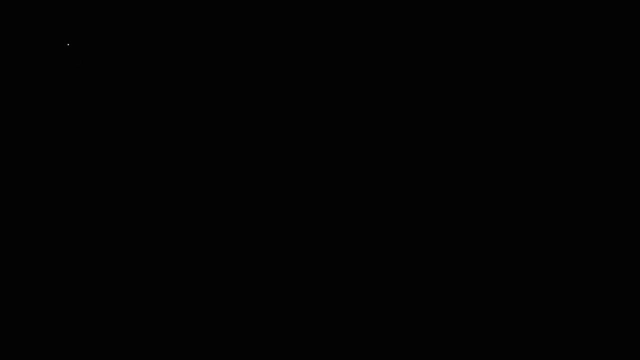 Let's do some more examples. So let's find a reciprocal of 4 and 3 over 7.. So first let's change this into an improper fraction. So we're going to rewrite the denominator, which is 7.. And then we're going to multiply 4 times 7, and then we're going to add 3 to it. 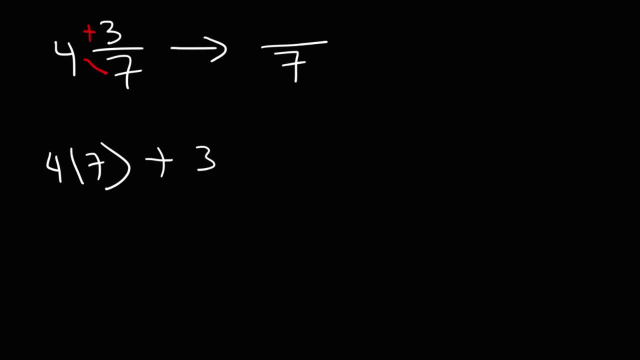 So that's 4 times 7 plus 3.. 4 times 7 is 28.. 28 plus 3 is equal to 31.. So this is 31 over 7.. Now to find a reciprocal of that, we are going to flip the fraction. 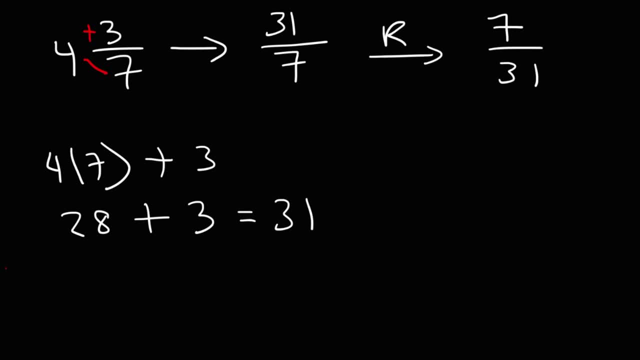 And so this becomes 7 over 31.. And thus this is the answer. Here's another one that you could try: Find a reciprocal of 5 and let's see 7 over 8.. Feel free to pause the video and try that example. 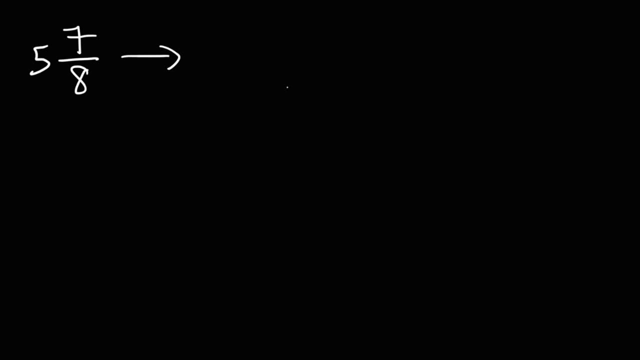 So let's turn this into an improper fraction. Let's begin by rewriting the 8. And then let's multiply 5 times 8, and then we'll add 7 to it. So 5 times 8 is 40.. 40 plus 7 is equal to 47.. 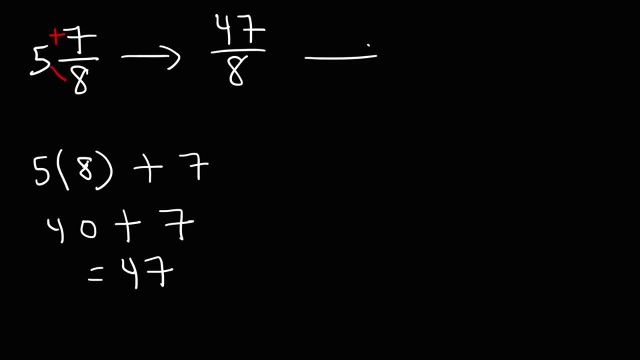 So this is 47 over 8.. Now let's find a reciprocal. So, flipping the fraction, this becomes 8 over 47.. And that is the answer for this one. Here's one more example. Try this one: 9 and 4 over 5.. 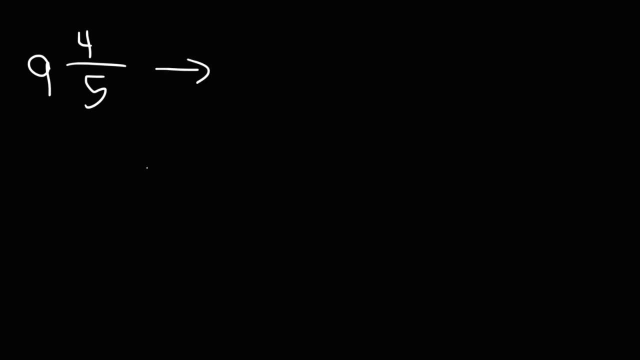 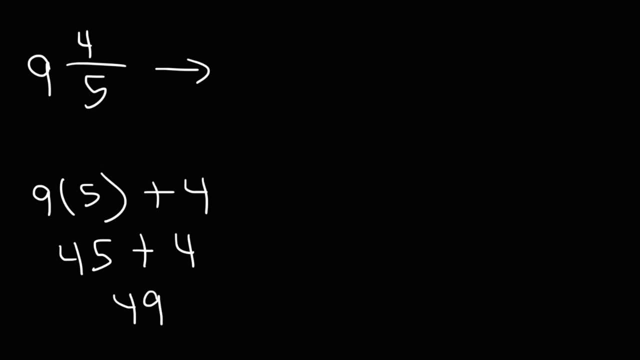 45 times 5 is 40.. 45 times 5 is 40.. 45 plus 4 is 49.. So this gives us 49 over 5 as an improper fraction, The reciprocal of 49 over 5 is going to be 5 over 49.. 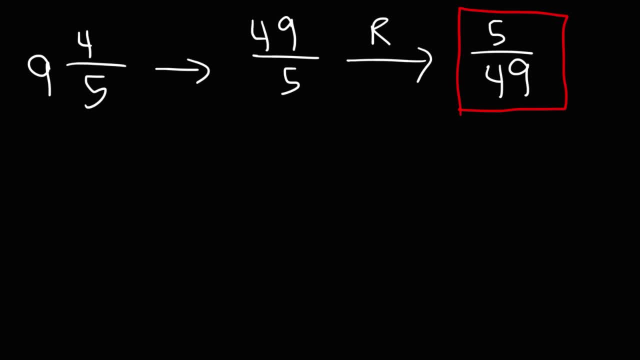 And that's it for this one. So now you know how to find the reciprocals of a mixed number. What about this one? Let's say, if you have an algebraic expression, A plus B, Divided by C minus D, 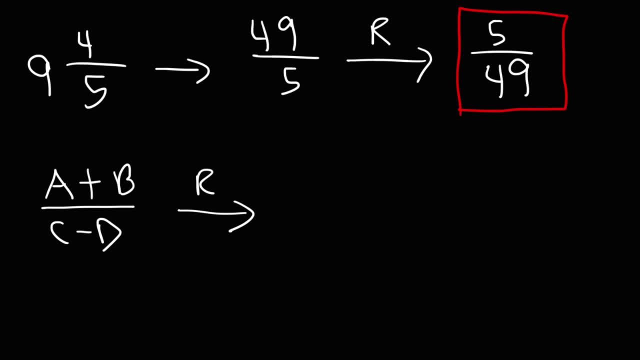 What is the reciprocal of that? Once again, all you need to do is just flip the fraction. So this is going to be C minus D over A plus B. Let's rewrite that again, And so that's the answer. So remember, in order to find the reciprocal of a fraction, just flip the fraction. 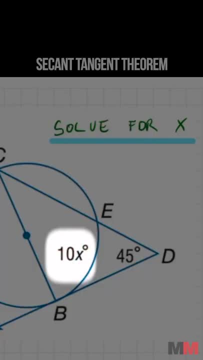 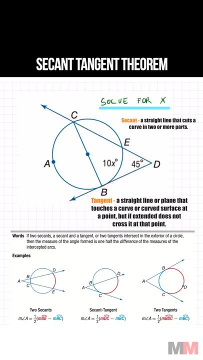 Here's a nice circle question for you We're trying to solve for x. Thing you got to remember is that if you got a tangent line and a secant line that intersect in the exterior of a circle, then the measure of the angle formed, which is 45 degrees, is going to equal one half the. 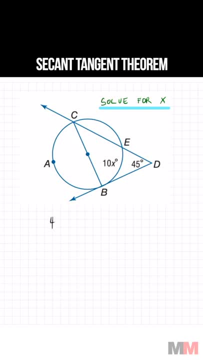 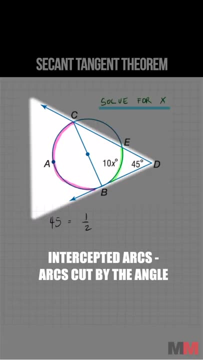 difference of the measure of the intercepted arcs, 45 degrees is going to equal one half the intercepted arcs. We got the big arc and the little arc, So we're just going to take the half of big arc which is not labeled. but this is a semicircle. You know that CAB is going to be. 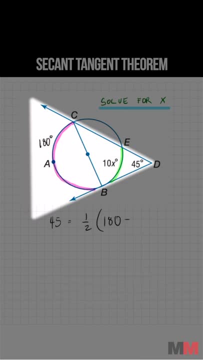 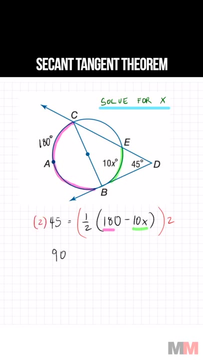 180 degrees, because that's half a circle minus 10x. Simple algebra from here. I like to multiply by two, just to get rid of the fraction. Now we got 90 equals 180 minus 10x. Subtract 180 and divide by negative 10.. X is going to equal nine degrees. Like and subscribe and I'll see you on. 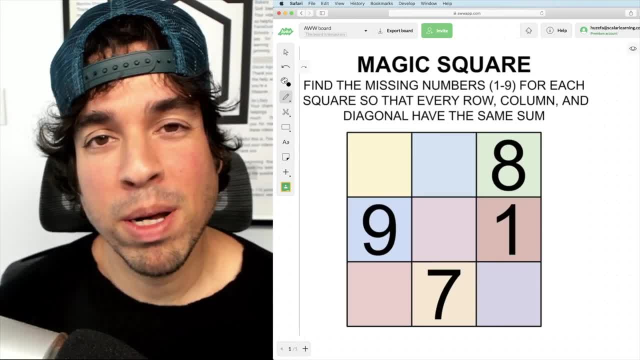 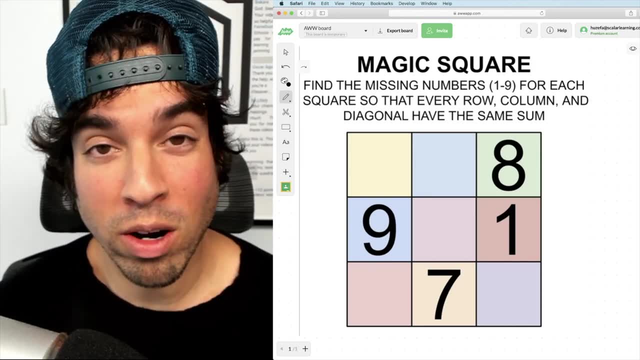 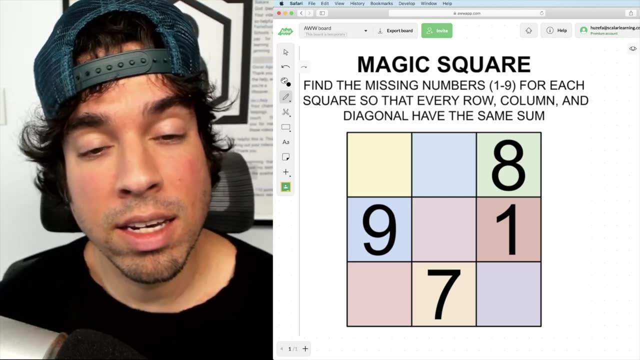 What's up everybody and welcome back to another math puzzle. This one is all about magic squares. So what are magic squares? Magic squares are these three by three squares where every single little square has a unique value between one and nine. Now the key is that you figure out all the